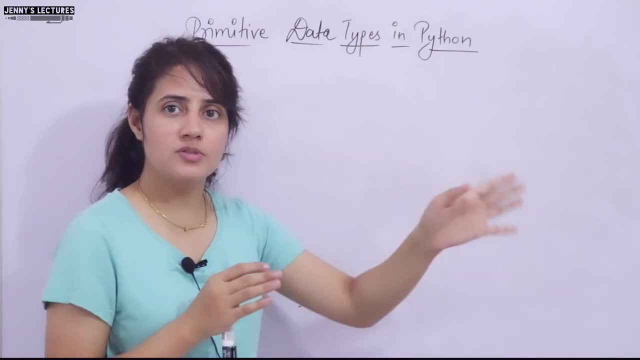 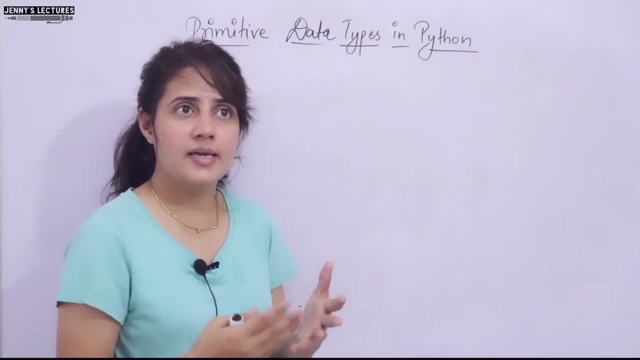 This kind of thing, But in Python it is different from C and C++, those languages In Python. Python is an object oriented programming language, so everything is like considered as an object. So in this case these datatypes are considered as classes. These are classes and the variable. 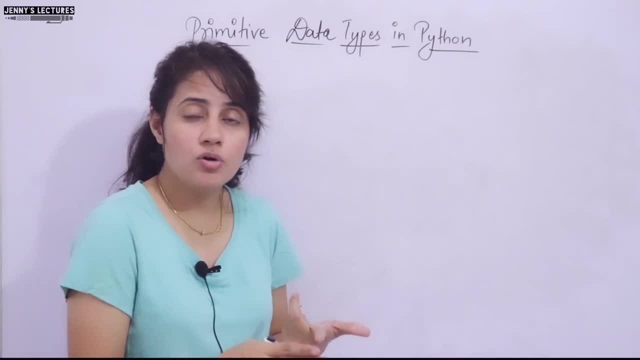 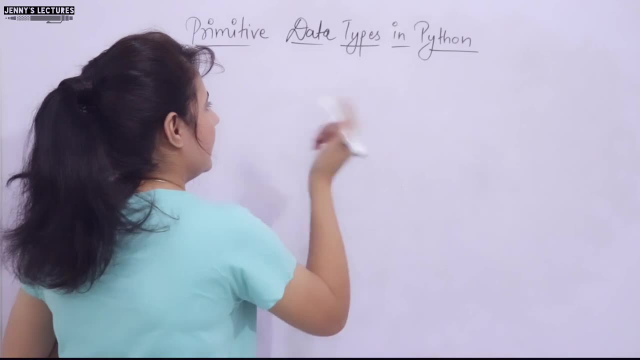 you create. those are known as instance or objects of these classes. Didn't get it? It's okay. Let me give you a quick example. Let me give you a quick example. Let me give you a quick example. Let me give you an example. If you write have to declare a variable, we write: 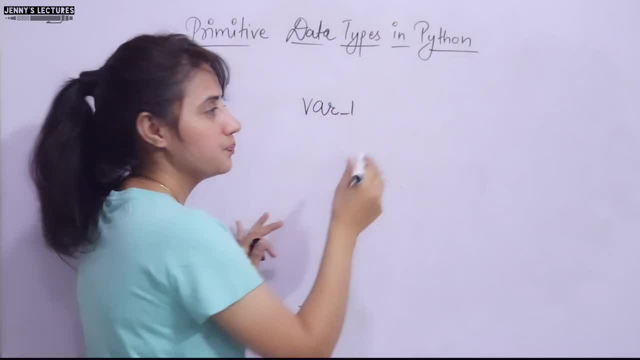 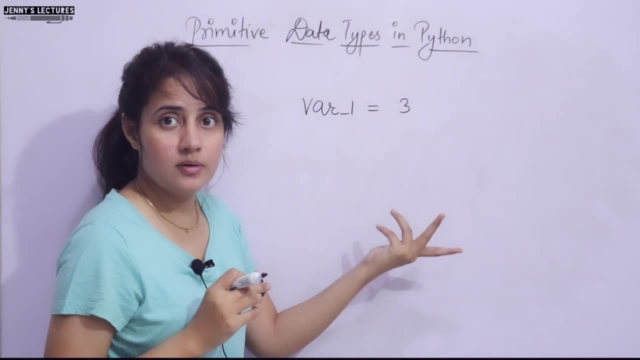 variable name, suppose I am taking variable underscore 1 equal to 3.. Now we know that this 3 is integer: whole number, whole number. so this variable of type, datatype of this variable is integer. Okay, So now, in this case, in this case, yeah, okay, the datatype. 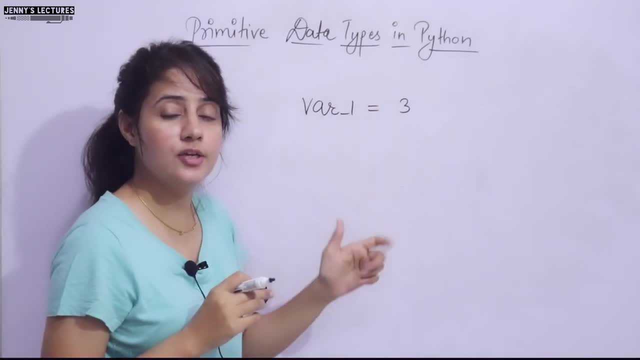 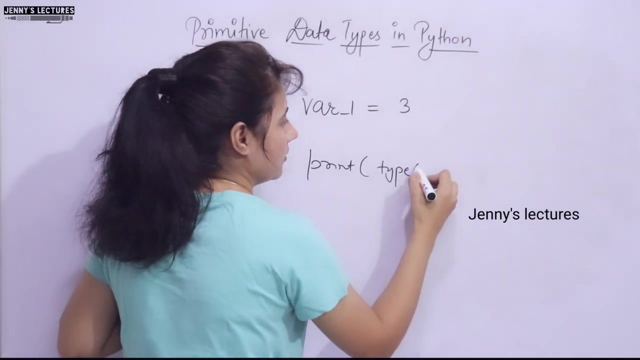 of this integer is. this variable is integer. But if you check the datatype in Python, we have a function to check the datatype of any variable. Okay, Have to check, we have a function type. So if I print something like this print type and within this type, I will be using this variable name var underscore 1.. So this: 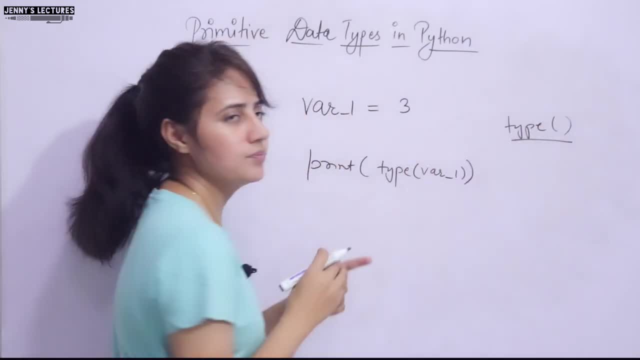 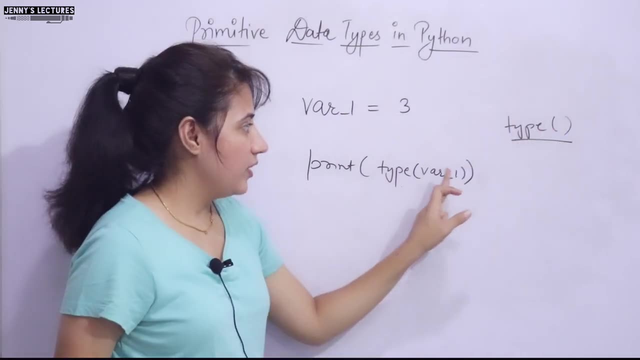 function type. it is used to check the type, datatype of a variable. Whatever variable you want to check, those you can write down here. Okay, So the variable I am writing var 1, so it will check the type and I want to print that. 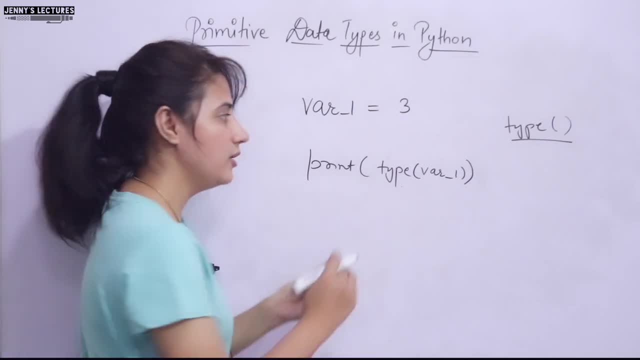 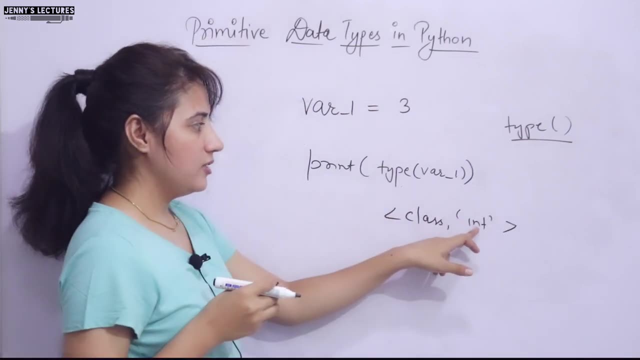 type. So that is why I am writing this function into print, So it will print what This kind of output you will get: class and int. So yeah, it is of integer type, but this int is what a class? So these datatype, these datatype like int, float, string, these are classes. 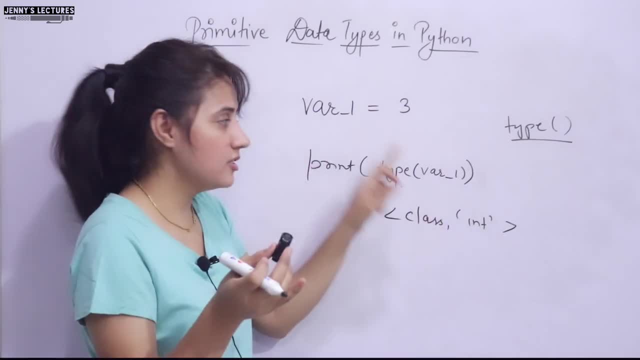 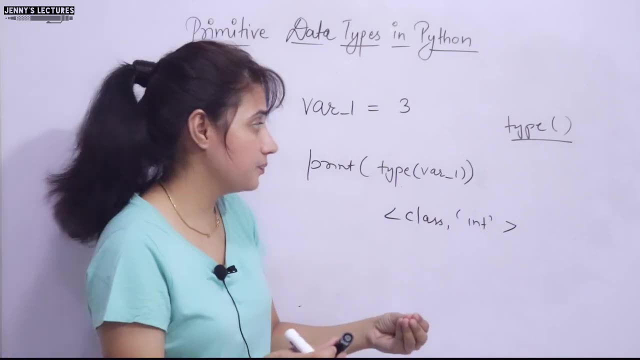 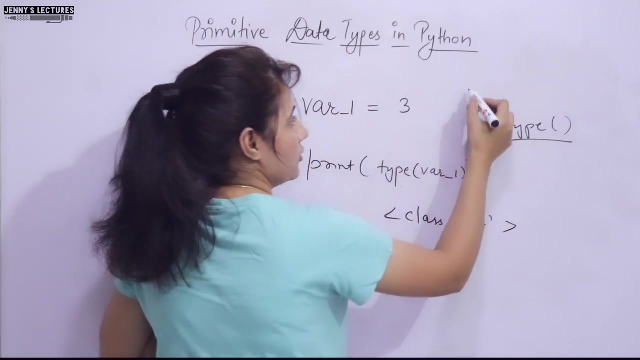 and now this var 1 is what Object or, you can say, instance of this class, int. So this is the case in Python Actually. Okay, This is actually the datatype in Python Right Now. see, in Python actually we don't need to tell like the name of the variable, Like in C or C++, we use int If 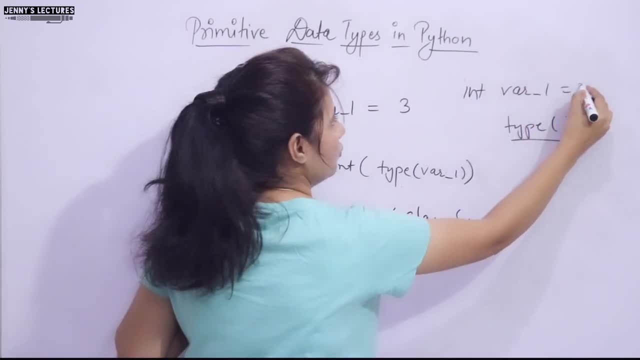 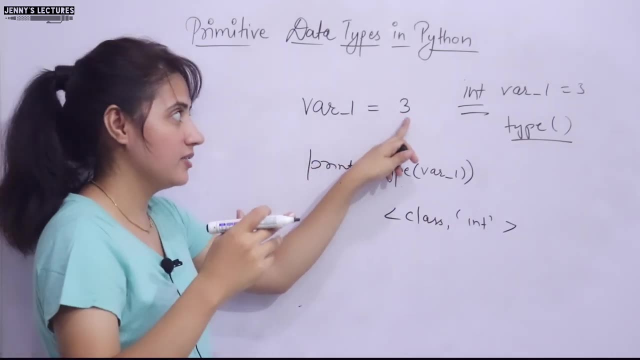 you have to write. then we write: int: var, underscore 1 is equal to 3.. You have to tell the datatype. But here we don't need to tell the type of the data. We simply write down the name of the variable. assignment: assign a value. Python itself will figure out the type of 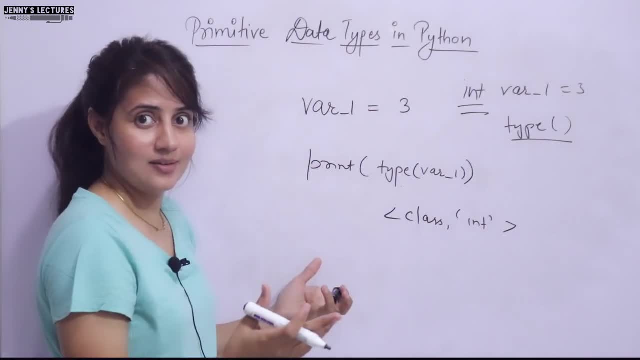 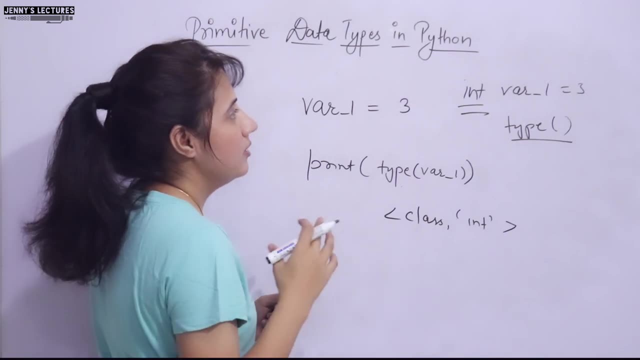 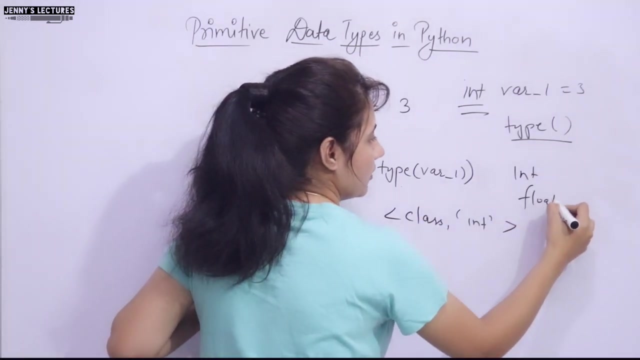 this data. Okay, That is a plus point in Python. Okay, Now see if I write something like this. So there are multiple datatypes in Python, Multiple built-in datatypes in Python. Basically in this video we will discuss int, float, string and boolean. There are multiple datatypes. 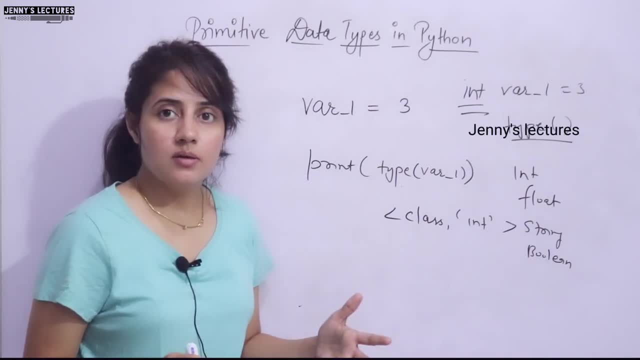 also List range, tuple, dictionary, set Right Complex. So those are also. we will be discussing one by one. Okay, So this is a plus point in Python. Okay, Now see if I write something like this. So 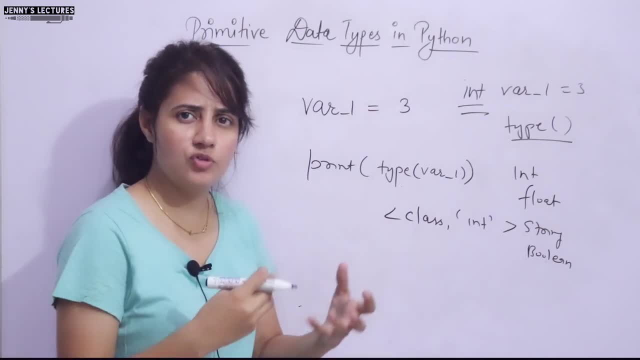 there are multiple datatypes in Python. Okay, So this is a plus point in Python. Okay, So, these are some basic datatypes. We will, you know, generally, mostly we will use these kind of datatype. So these things, these 4 datatype, we will discuss in this video. 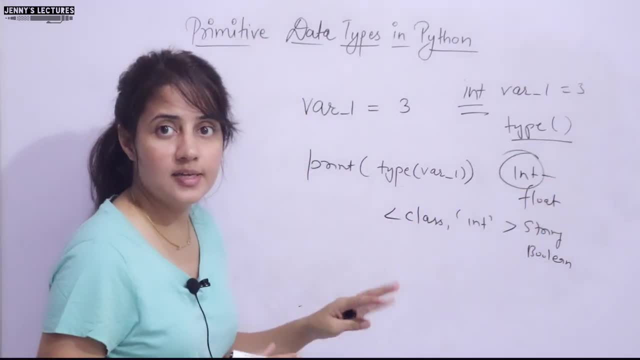 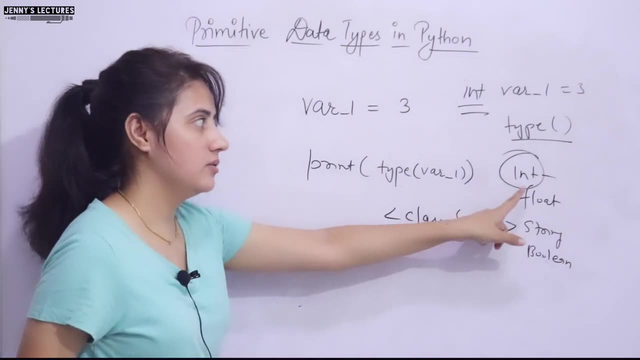 Okay, Now int. So int will. this is what contains integer, like whole number. it will contain, from positive to negative, Any number. and one more thing: there is no range the number, There is no limit on the number. You can take the number as long as possible, Although the 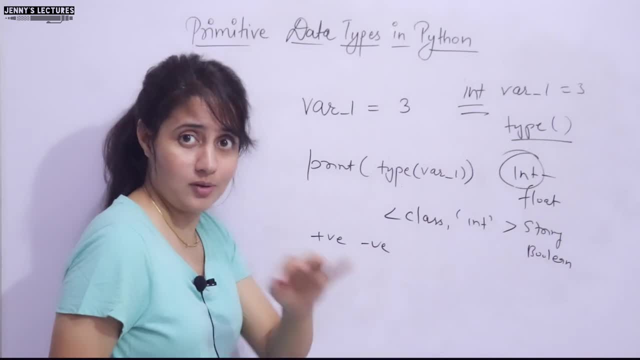 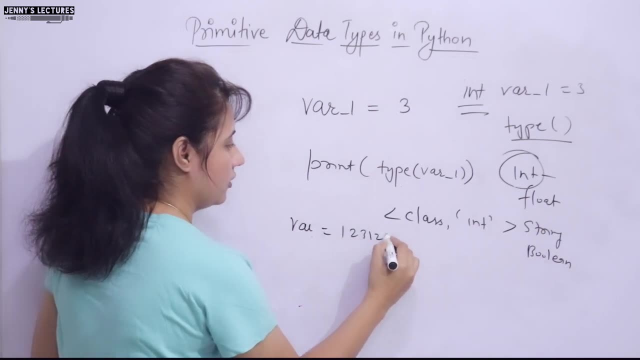 construction is there, Although the constraint is your memory of your system. If I write something like this, if I am taking a variable where is equal to 1,, 2, 3, 1, 2, 1, 2,, 1, 2, means a long number I am having. yeah, it is possible to take a long number. 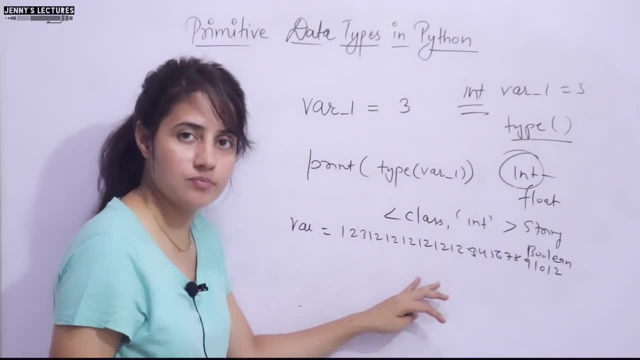 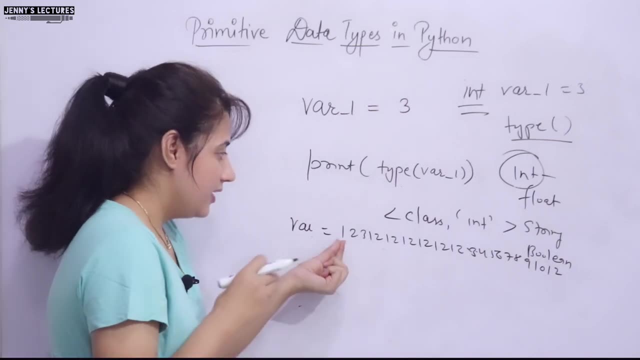 and you will print the number. then you will see this number would be printed. okay, But see this: if you go in more deep, let's discuss in more deep. actually, if the number is without prefix, then that would be considered. the sequence of decimal would be considered. 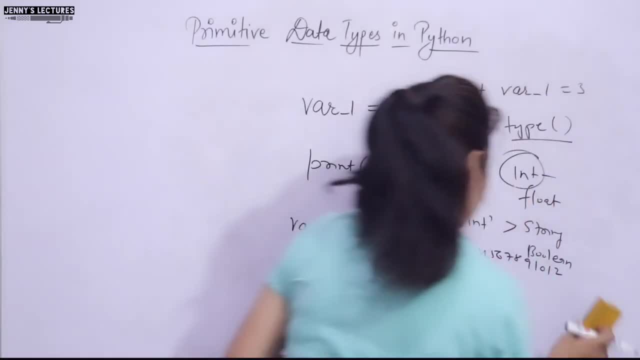 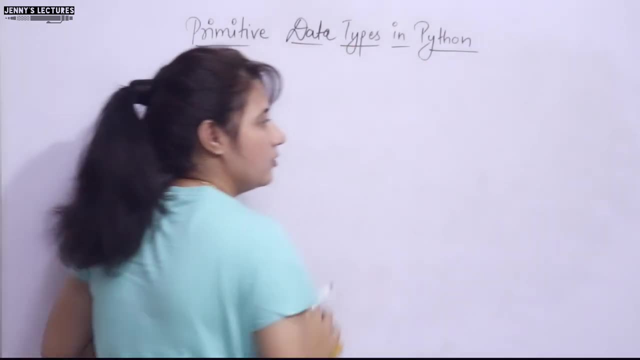 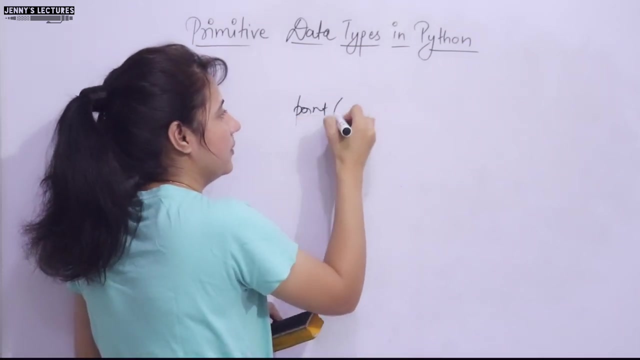 as a decimal number. If you write here prefix, what prefix? we can write Something like this: see, as we know, decimal number or integer can be of binary type, octal type, hexadecimal type. okay, So if I write a number, something like this, if I print something like this: print 0 and. 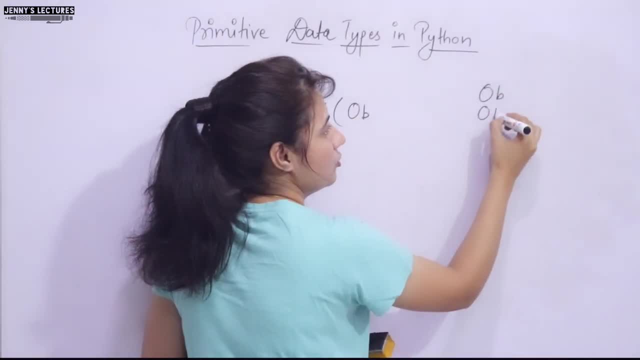 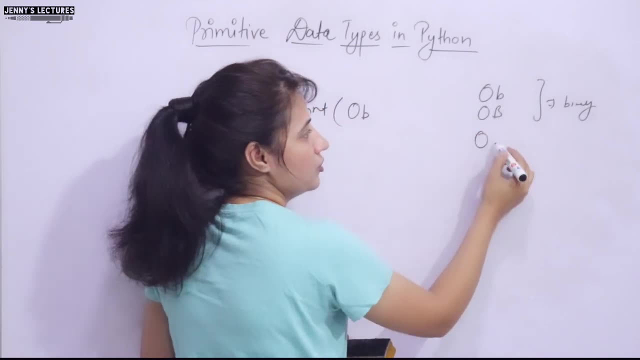 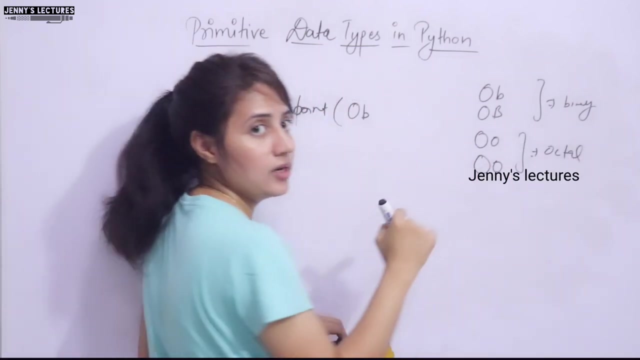 b. see this prefix, 0 b or 0 capital B. This is for 0. 0,. this is 0, 0, small o, 0, capital O. this prefix is what For octal number. Octal numbers are actually prefixed with this thing: 0, x and 0 capital X, small x, capital. 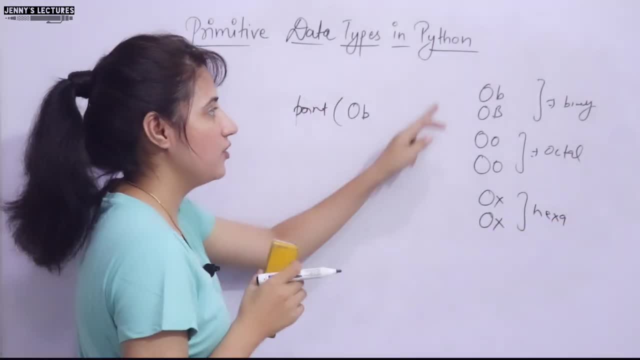 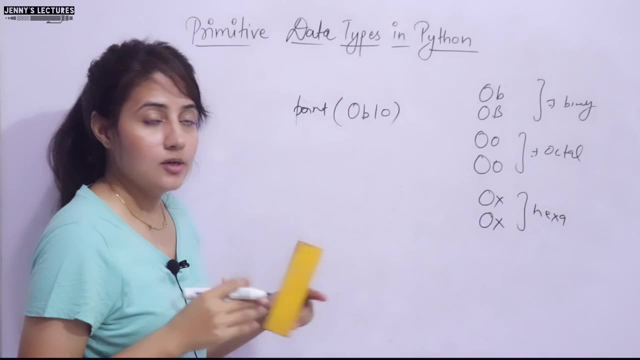 X. This is what This is, a hexadecimal number. So if a number is prefixed with these things, like I am writing a number 0 b and I am writing 1, 0, 0 b means 0 b or capital B. 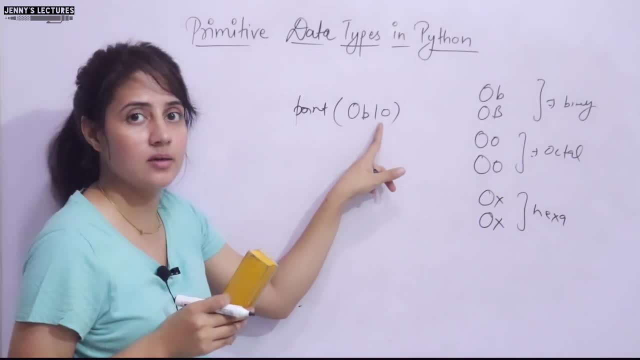 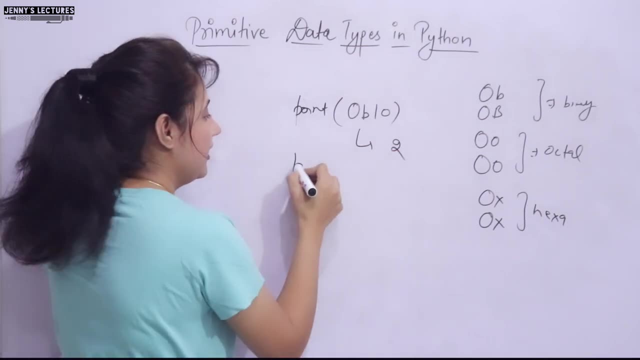 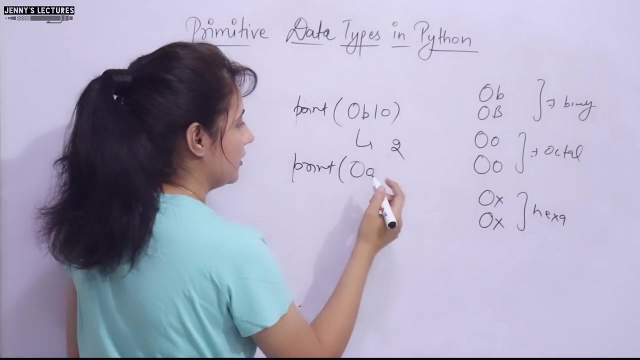 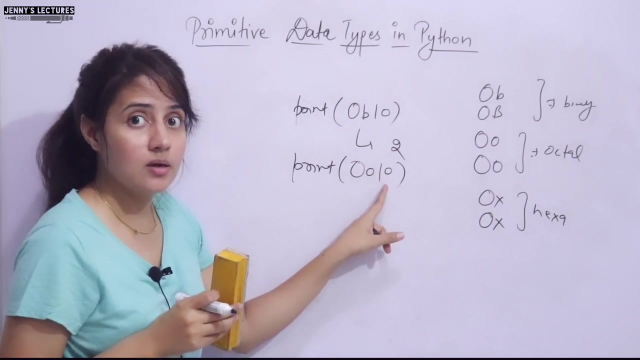 Now compiler would interpret that this is binary number means binary 10.. Binary 10 means in decimal it will print 2, fine, If I write something like this: print 0 and small o or capital O, and I am writing something like this, like here, I am writing suppose 10, so 0, x prefix means it is octal number. 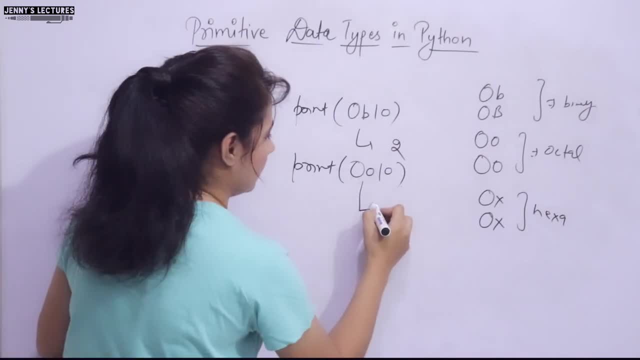 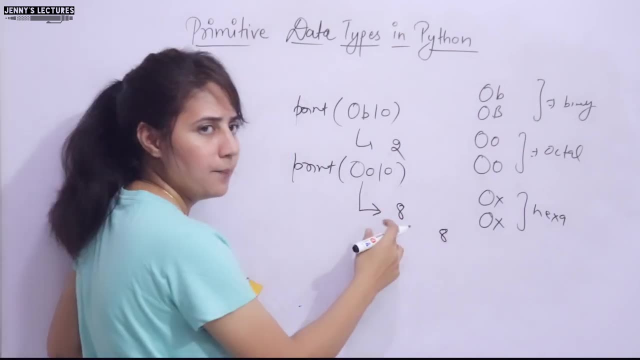 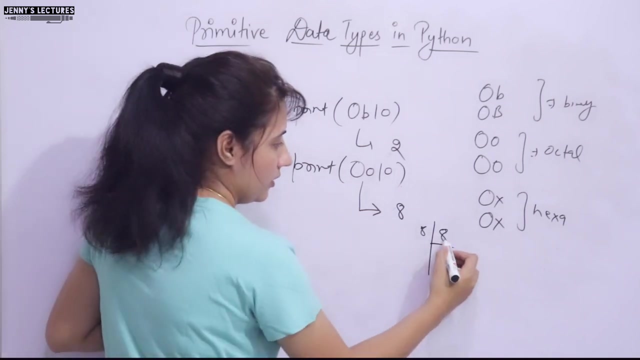 So the equivalent number, decimal number. So this is what I guess: 8, decimal number is 8.. If you are not sure, you can convert. like if I have decimal number 8 and I want to convert it into an octal number or base 8, so you just have to divide it by 8,: 8, 1, 0, 8 0, 1.. 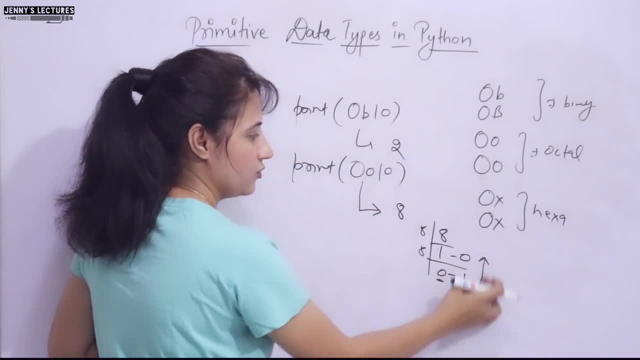 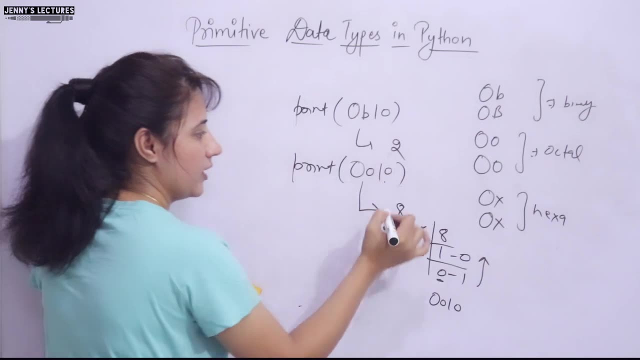 Once you get 0,, stop and just write down these digits from here to here: 1, 0,, 1, 0.. Yeah, The octal of this 8 is what? 0 o, 1, 0.. Yeah, That is 8.. 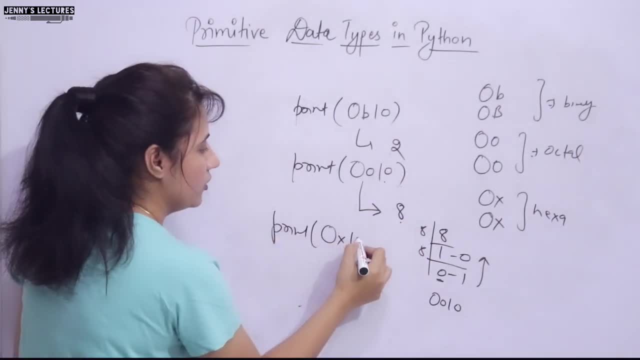 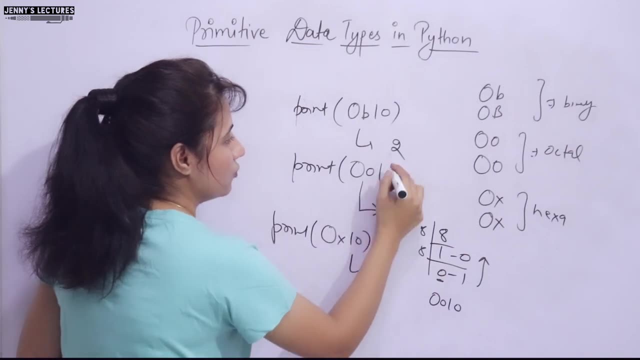 If I write something like this: print 0 x, 1, 0, it will print, I guess, 16.. If you write, rather than 1, 0,, if I write something like this: 1, 2, 3, it will print what? 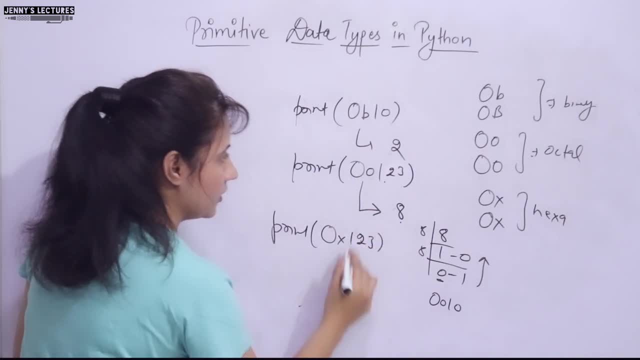 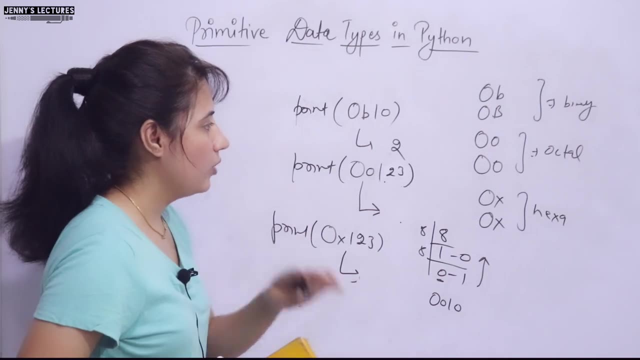 And if I write 0, x, 1, 2, 3, so you have to try this out. This is octal number, this is hexadecimal because it is prefixed with this. So what decimal number you will get? what decimal number you will get? 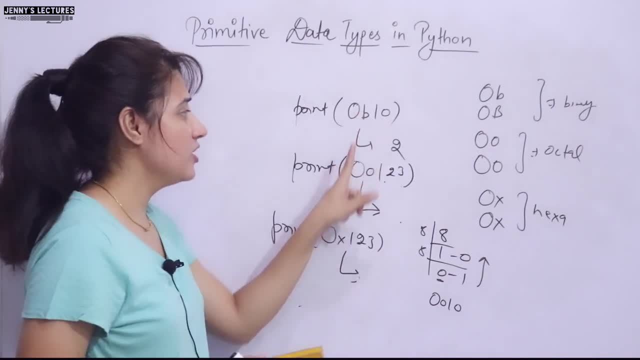 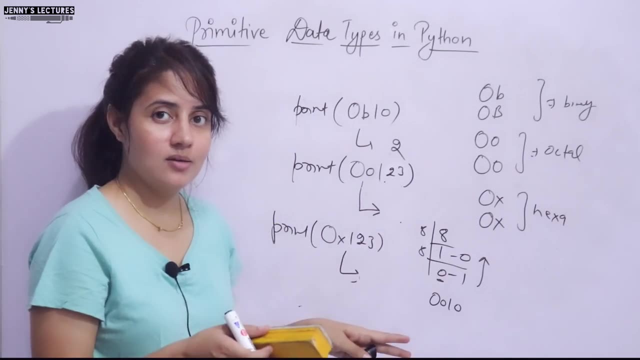 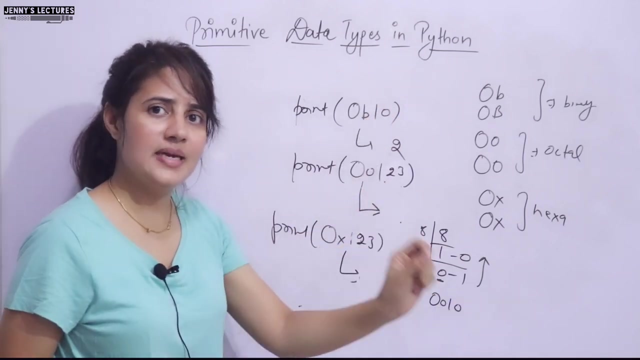 You have to figure it out, you have to tell me in comment section. So if the number is prefixed with something, then that would have some different meaning. not, that is not a decimal number, that is not base 10.. Fine, But if you know, find out the type of these numbers also, then you will get. it is of type. 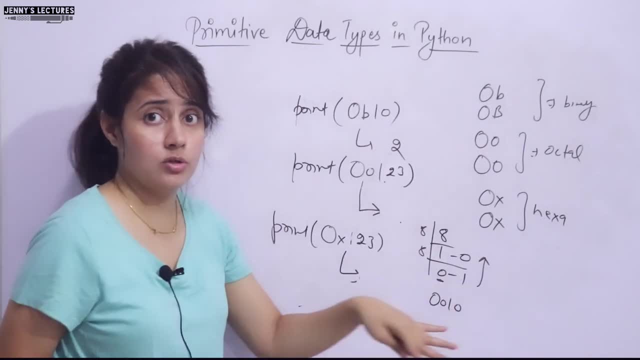 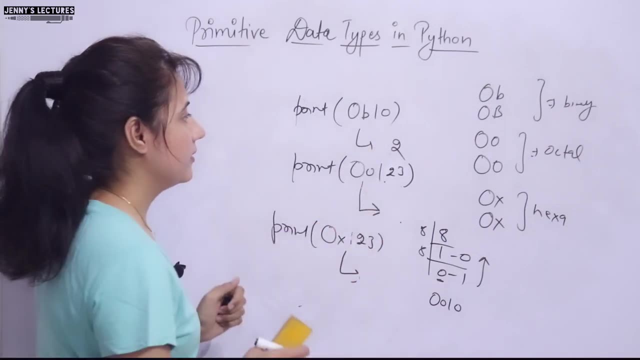 int. Okay, It is not like binary or octal or hexadecimal, These are parts, or you can say between, under this decimal number, under the integers, But the type would be int. Next is float number. So float is basically just decimal number. 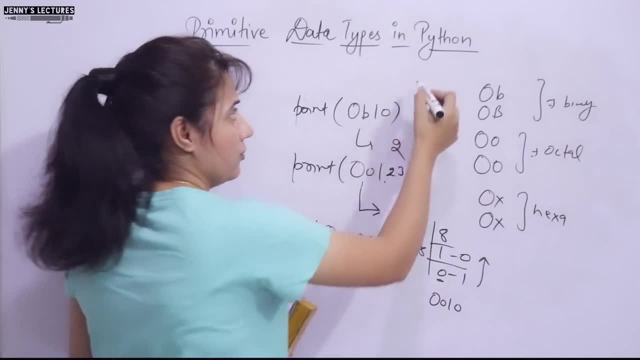 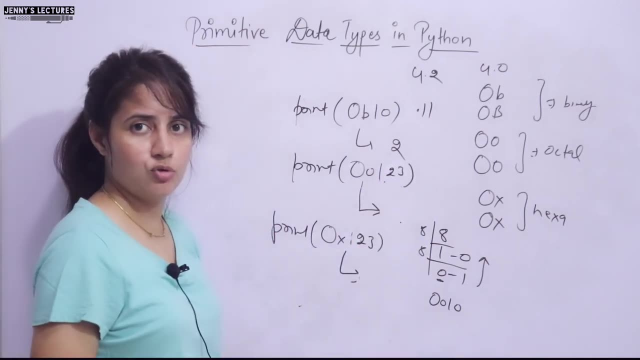 Yeah, So the decimal number or fraction we are having, those are float numbers, like I am having 4.2, 4.0, 0.11.. These are floating point number or scientifically, scientifically, you can denote with this E, notation E or capital E. with this thing also we can denote, but you don't have to go in. 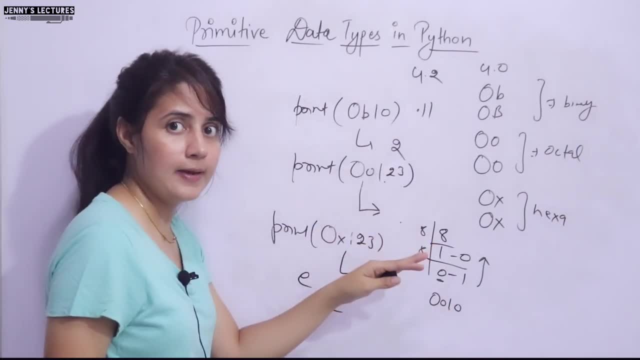 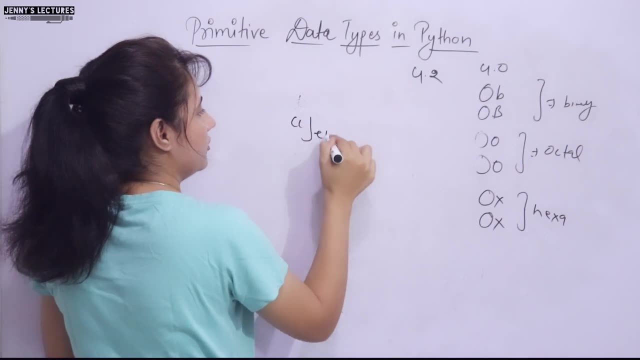 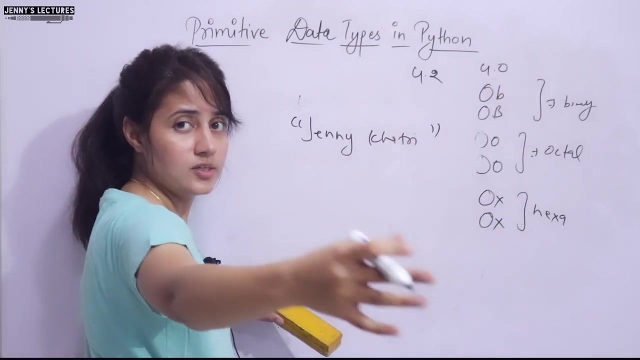 this much deep. Just you have an idea of it. it is float number. Okay, Strings. obviously sequence of characters are strings. So this is what string like I am writing Jenny Khatri or any like Jenny's lectures: CSIT, NetJRF, you are the best, this kind of thing. 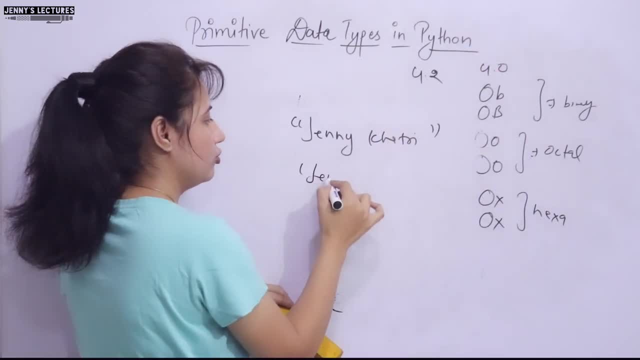 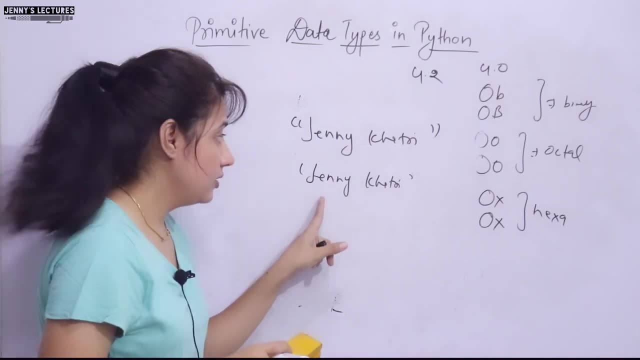 you can write. So this complete is what A string. or in single quote. also in Python we can write down string. We can now, you know, fetch individual character from the string using subscript. So I guess this thing will be seen practically. 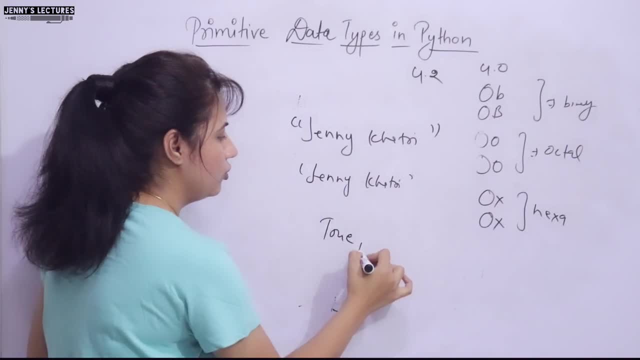 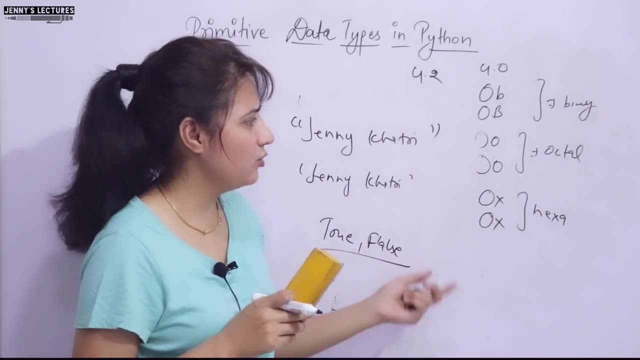 I hope now. next is Boolean. Boolean is what? True, Having only two value, true and false. How to use this? So let's just, you know, do some practical and we will see on our IDE how to use these data types and variables and all. 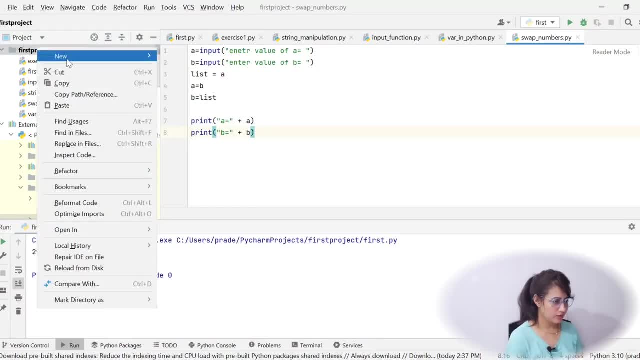 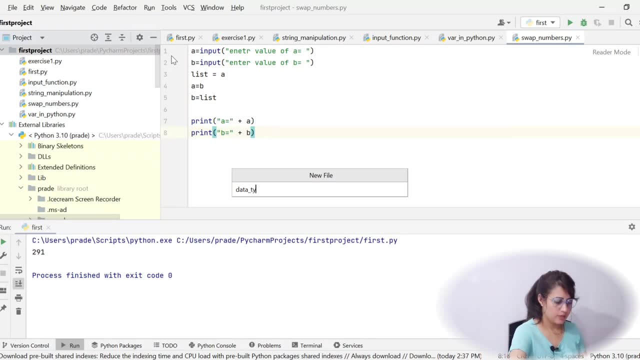 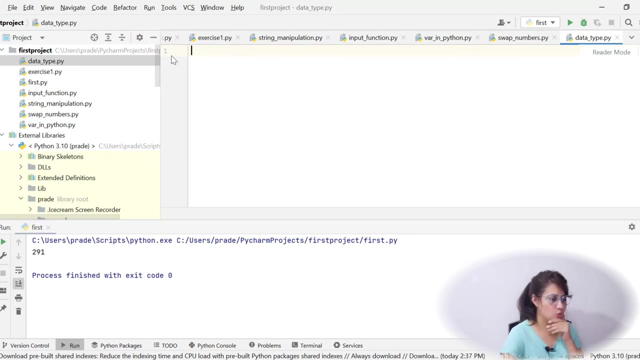 Okay, So let's create a new file. I am taking new file and we are taking the name: data, type: data, underscore type: dot, py. Okay Now, first we will take a variable. Suppose I am taking variable one, not hyphen, it's underscore one. 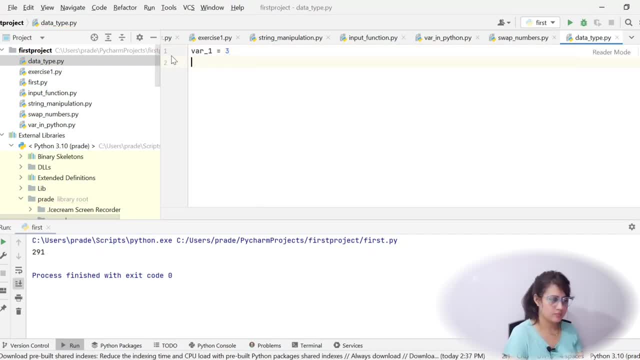 Variable one equal to. I am taking a value three or any value you can take, like one, two, three, four, five, six, seven, eight, nine, any long value we can take, Okay, And it will print. Suppose I am printing: print var underscore one. 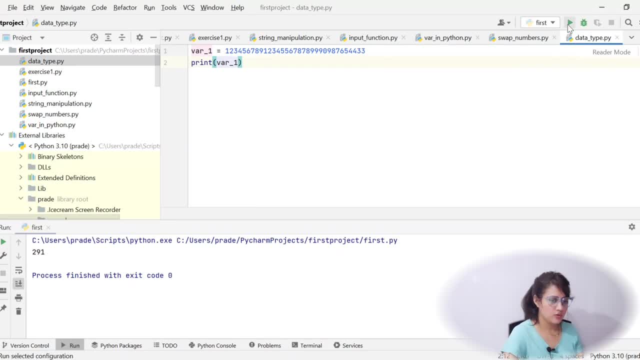 So let's run this and see what output you will get. Okay, So let's run this and see what output you will get here. Right click on this, right click on this space here and just run data underscore type: dot py- this file. 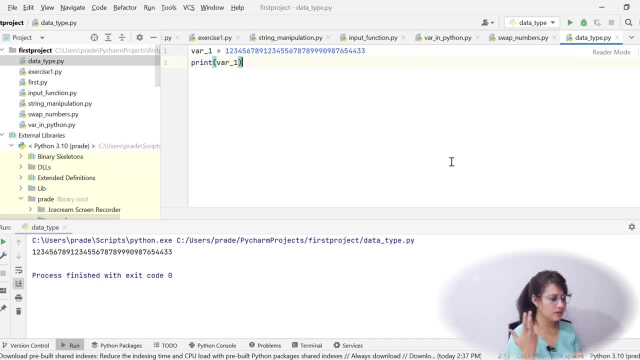 See, it is printing this number. So the number you can take, any long number you can take, there is no limit, there is no range in Python, but the limit is only the constraint is obviously the memory of your system. So some operation also like: if I do plus here one, that also fine. 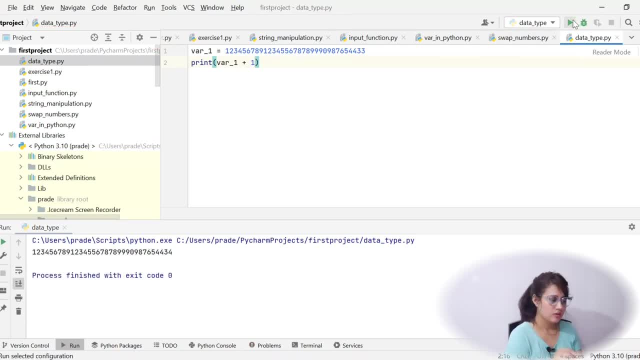 This plus will what It will just add. It's like addition. Two integer values are there. it will add one to this number. Okay, So if I am taking a number, something like this: one, two, three, and I am taking second, 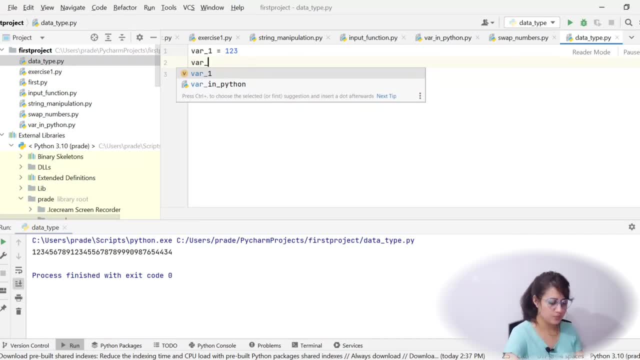 number var underscore two, and that I am taking like ten point one. Okay, So the second one is what Float? And if you want to check, if you want to check the type of these variables, then how you can check, Suppose I am concatenating these two numbers, var one underscore var two. 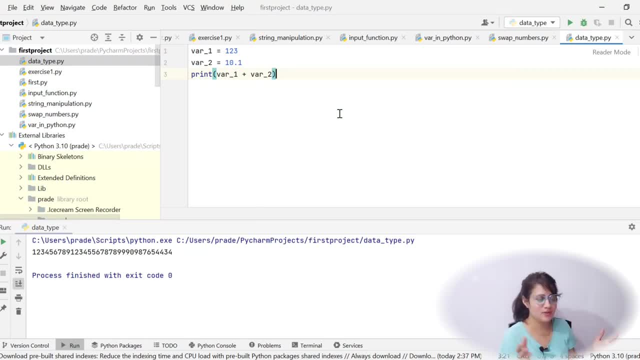 Concatenating means concatenation of strings are possible, but here this plus is what Addition I am adding these two numbers. So what would be the output? Let's run this: It's 123 would be added to 10 plus 10, point one. 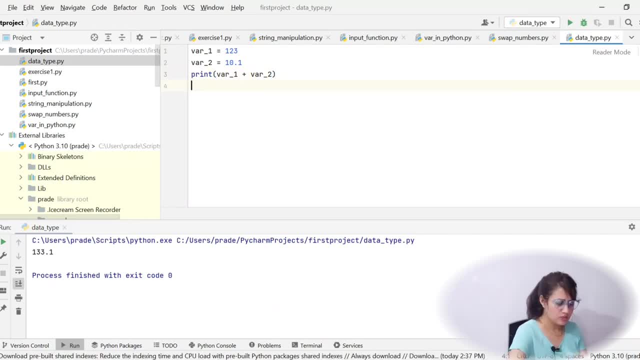 So 133, point one, If you want to check the type of these, so you can simply check the type with this type, function type, and I am checking the type of var one- Okay, And obviously you will print what is the type. So for that we have to use print function. 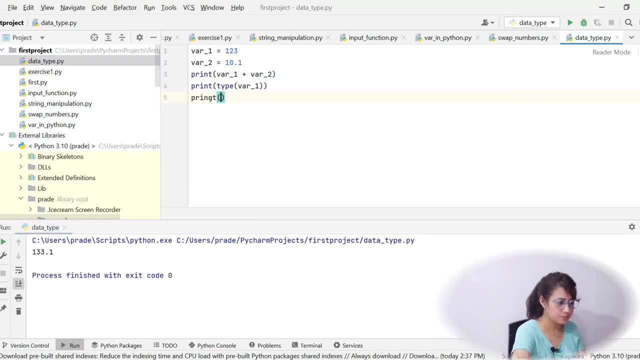 Again, I am printing like print Okay, Type and var two, this variable. So let's run this and we will see what output you will get. Okay, This: there is a name error, See name error. One more error we got: 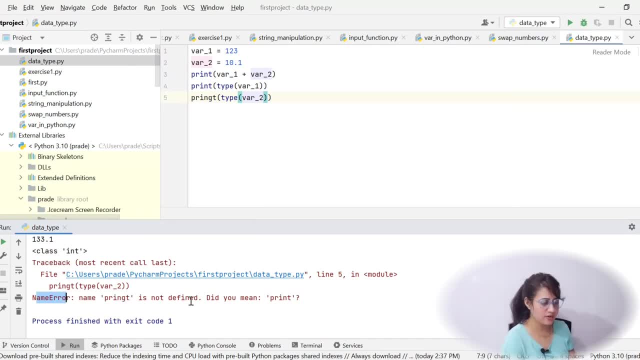 Print p, r, i n g t is not defined. Did you mean print? Yeah, If you have done something like this, it is not syntax error, It is a name error. Okay, So there are types of error also, So let's correct the name. 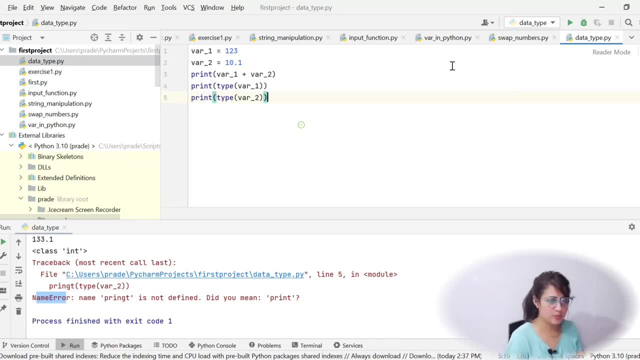 It is print. And now let's run the C. You can see this: first the addition. then for var one, it is of int class class is int and var two class is float. Okay, So these data types are actually classes in Python and these variables are. you can say: 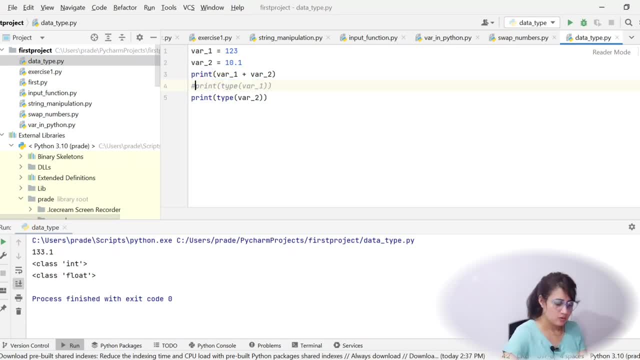 what objects of these classes. So let's comment this out and see if I route with prefix. something like this: If I want to add this prefix, 0 and o, Okay, Okay. And if I print the value var underscore, 1,, 0 means it is octal and in var two I am taking 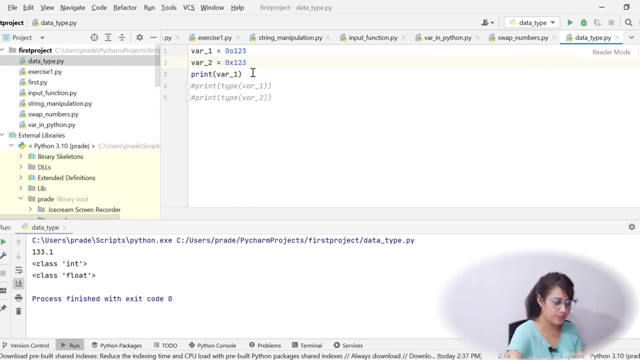 0 x, 1, 2, 3, and I am printing var 2.. So let's see what it will print. First, output is 83.. So 83, if you convert 83 into octal, you will get 1 to 3.. 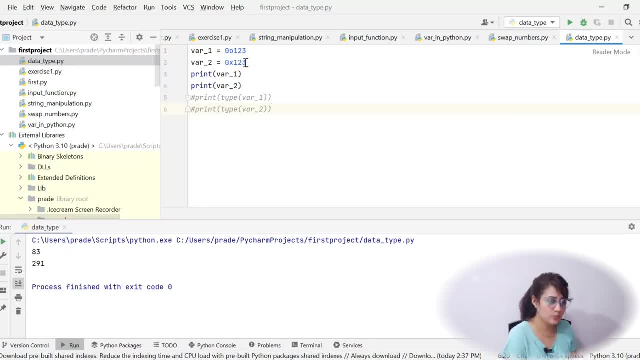 If you convert 291 into 3,, you will get 1 to 3.. Okay, If you convert 28 to 23,, you will get 0.. So, if you convert 28 to 23,, you will get 1 to 3.. 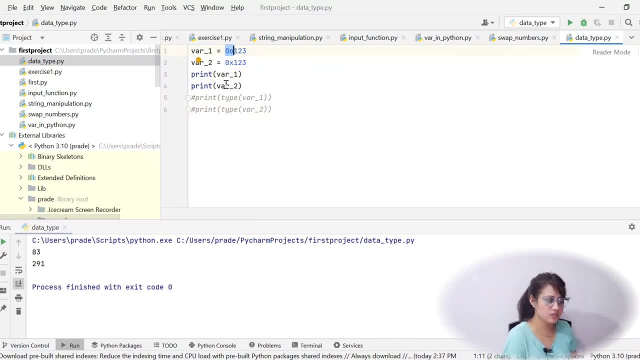 So with prefix you got some different answer. These are not considered as decimal number, but with prefix they you will get some different result. And simply without prefix, if you print like var, 3,. let's take a another variable: 1,, 2,. 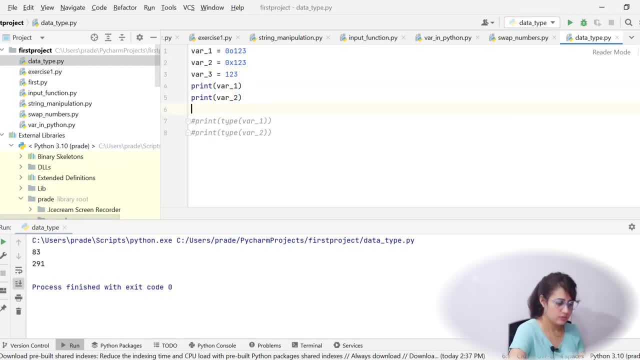 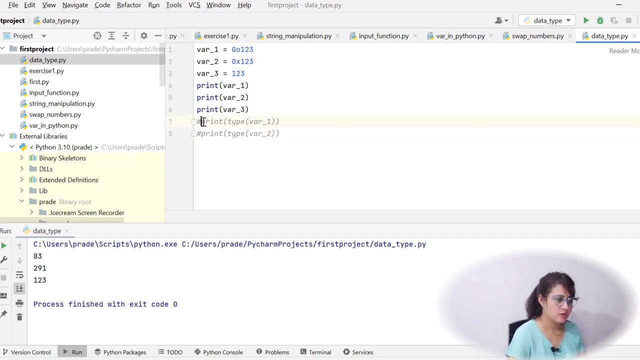 3 and just print var 3.. So without prefix. obviously it is decimal number. So it will print 1,, 2,, 3 only. and if you check, now you check, if you check these type of variable 1 and 2, then what you will get int only, int, int. obviously with prefix. interpretation is: 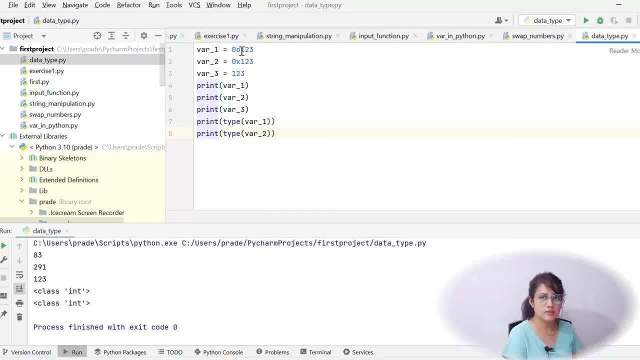 this is, this is octal, this is hexadecimal, but these are of int class or int time. Okay, now let's float number. we have seen, like what a float number. let's have strings. So I am having, like I am having, a variable name name, and there I am having jenny khatri. 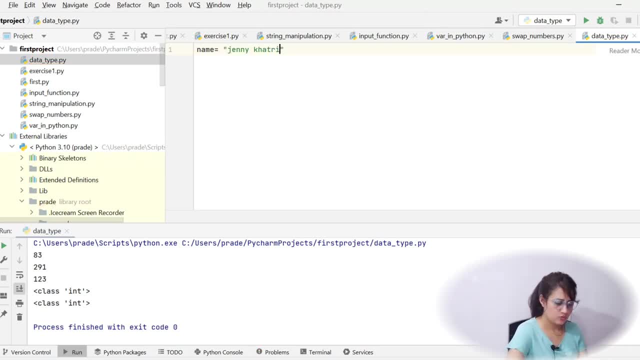 in double quote or single quote you can use. So if you simply print, first, let's print type of this thing. If you print type, then the class is str. for string type, The class is str. the data type is str, the class is str. and if you print this name, obviously 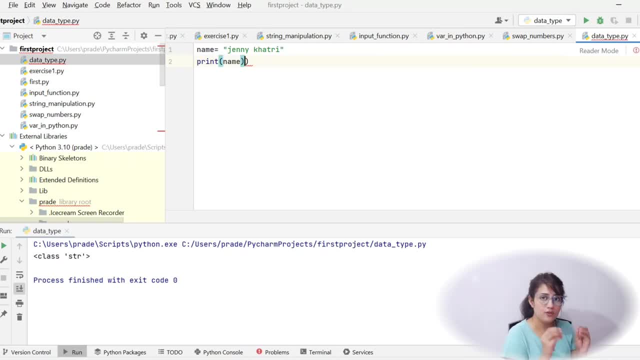 you will print here jenny khatri. but you can fetch specific characters with subscript. If I write name and in subscript I am writing 0, so what it will print? j see it will print j. now you will get j because it is sequence of characters, so it would be stored as array. 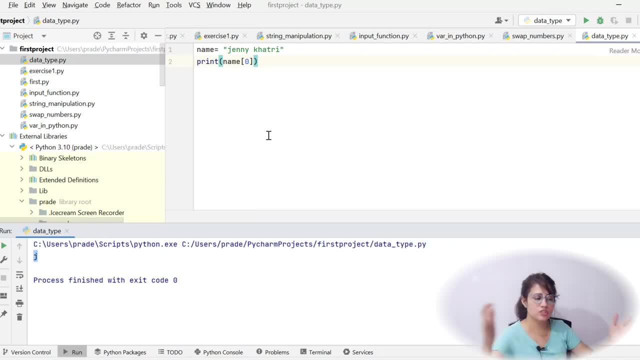 like the index would be started from 0.. 0, 1, 2, 3, something like this. and if I print something like this, see if I print 0, 5. so let's post this and try this out- what you will get at 5. now let's run this and see you. 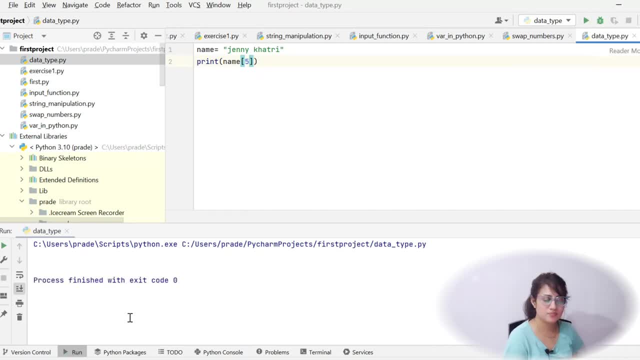 will get nothing because at 5 index there is space. if I print here 7, then you will get h, so you will get h here. okay, so subscript also possible, like you can access every character of the String and if I am writing here something like this, like name and name, underscore 1. 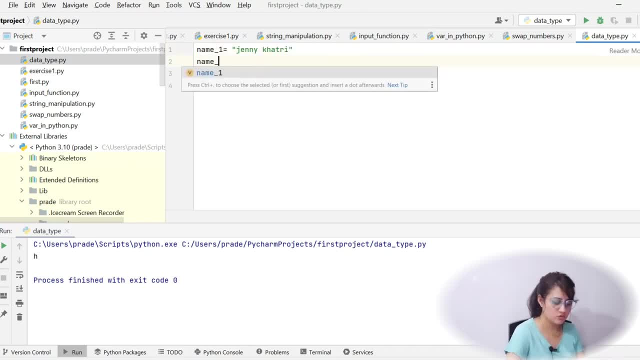 name underscore 2. one more variable: I am taking name underscore 2 and there I am writing jenny khatri and here I am writing cs, faculty, computer science faculty. and I am just adding, sorry, something: name 1 plus name underscore 2, so obviously it will do concatenation of these. 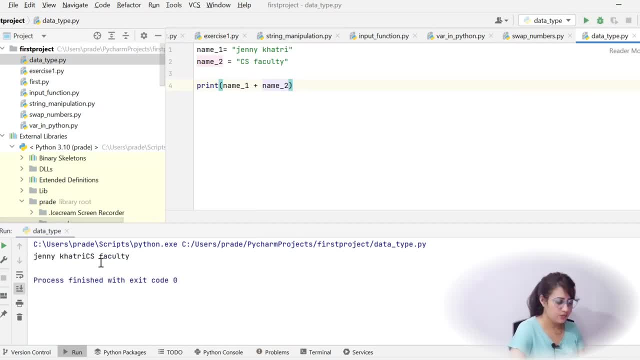 jenny khatri with no, no space, cs faculty: okay, but see, if you take a variable variable- or I am taking here a- a is equal to 1 and if I write something like this name- 1 plus a- in this case it will give error. see, it will give type error, not syntax error, it's type. 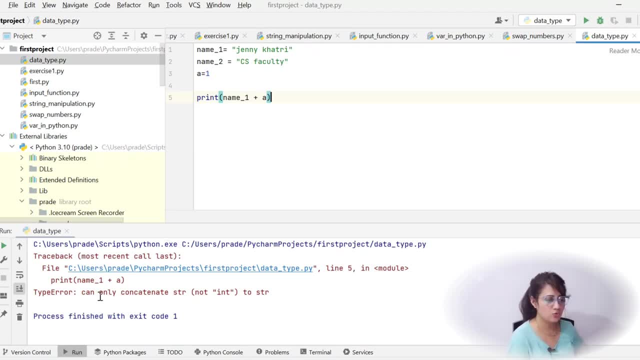 error Can only concatenate string- Okay, Not int- to str, because name 1 is str and a is what integer. so we cannot concatenate these things. so you have to be very careful while you using these data types, because these are, you know, they have they having their own properties, some functionality, some functions and all so. 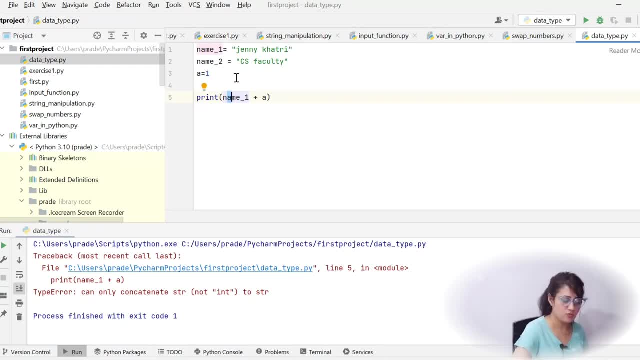 this is not possible. but if in name 1, if in name 1, or you can say here I am writing name 1 is equal to 1, 2, 3, still, still. if I run this you will get an error because 1, 2, 3 it's. 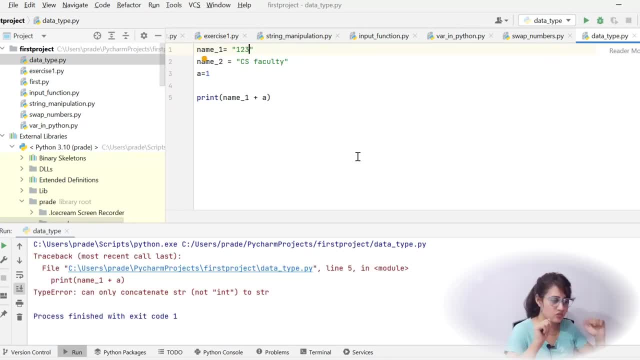 not integer. you are putting double quote here, so it is a string. so it is not possible here. but 1, 2, 3, name 1 plus name, underscore 2. and suppose, in name 2 I am writing see, in name 2 I am writing 1, and we are doing name 1 plus name 2. so what do you think? what do you think? 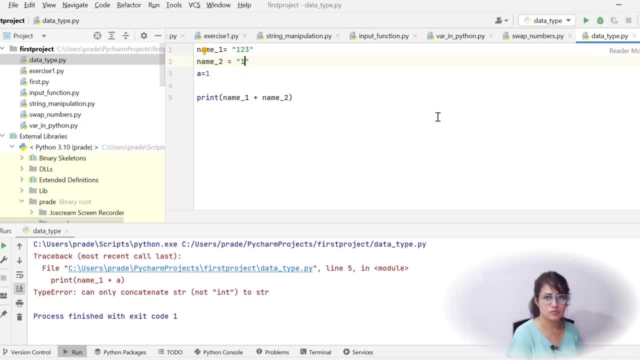 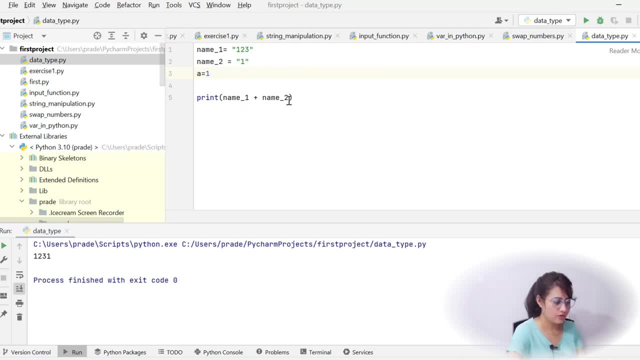 than this. if I write something like this: 1, 1, 2, 3 plus 1, now these are obviously integers, so you will get 1, 2, 4 and here, obviously, if you put here also these, these thing, obviously these are string after putting these codes. so 1, 2, 3, 1, you will get here. 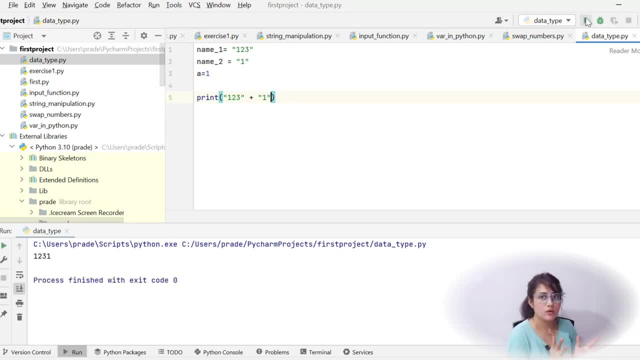 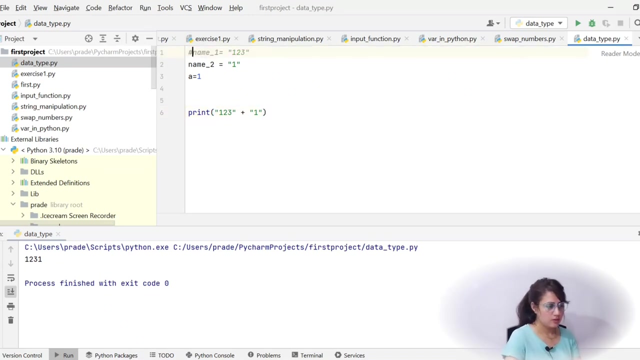 so you have to be- you know- very careful about using, you know, when you use these data types. what is string? what are? anything you will write in single code or double code, whether it's a number or characters or anything that could be considered as string. okay, now let's just comment these out and sorry, and this we 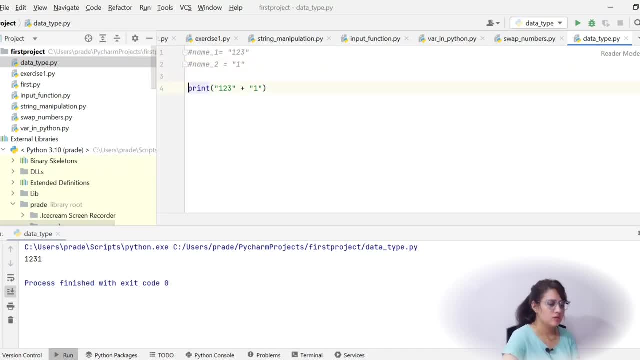 don't want and in print I'm writing what I want to print Jenny's lectures like in this way: Jenny's lectures. okay, that will print Jenny's lectures. no doubt because we are printing the single code but out of the outer side we are using double codes. so within you can use single code. that is fine. okay, Jenny's. 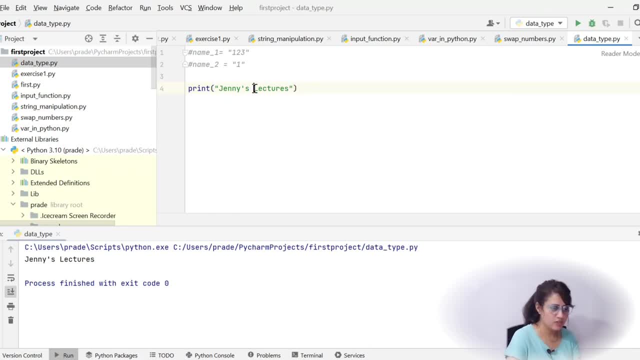 lecture. it is printed, but suppose I want to print Jenny's and lectures in double codes. so now both. I want to print single code as well as double code on the screen. so what to put out aside? we cannot put single code, we cannot put double code. now what is the? 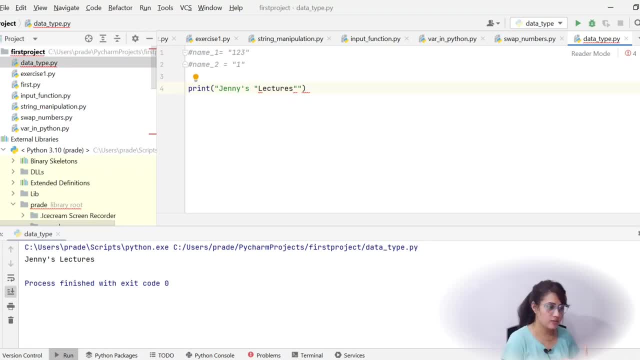 solution. so in this case you see the single code. these double codes are having some obviously special meaning to this interpreter, this Python. so if you skip this special meaning, we can do a task. so yeah, there is a way. this- a special meaning of these single code and double code can be skipped, in which way you have to use one forward. 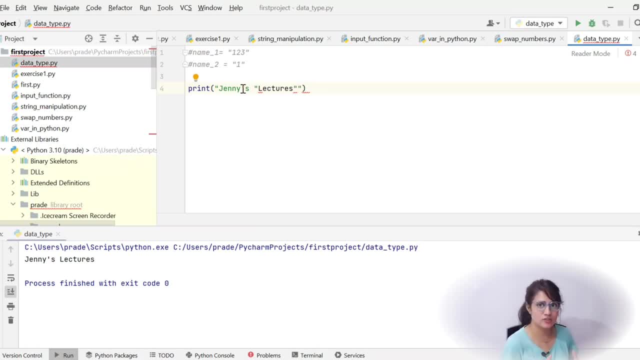 slash, sorry, backward. slash, backslash, you can say backslash. so before this single code, use this backslash, before this double codes. also, because I want to skip the special meaning of this, use this backslash before this. use this backslash. ok, now this is what you can say. skip sequence, we will. 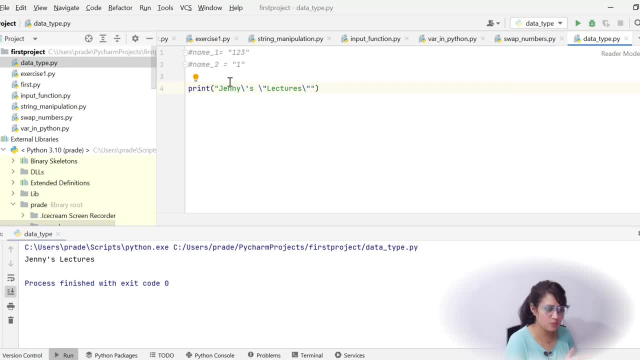 discuss these things later, in later videos. so we are going to escape, we are going to skip the special meaning of these quotes. now it will work fine. see, now let me just run this and it will print jenny's apostrophe single quotes and lectures in double quotes. 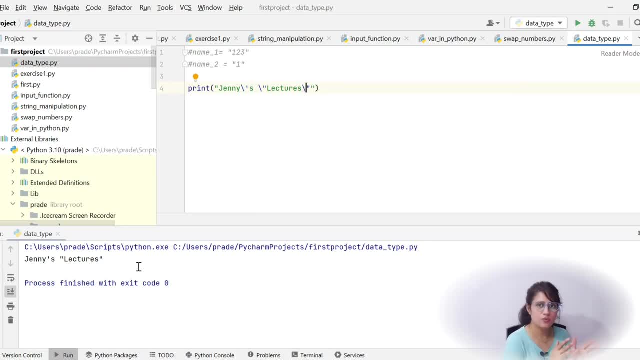 so we are not getting any error. so if you wanna skip the meaning of anything, any special meaning of these, you know symbols and all- you just use a backslash. that is it? ok, like suppose here I wanna I jenny's, and after that I have put slash n. ok, let's just run. 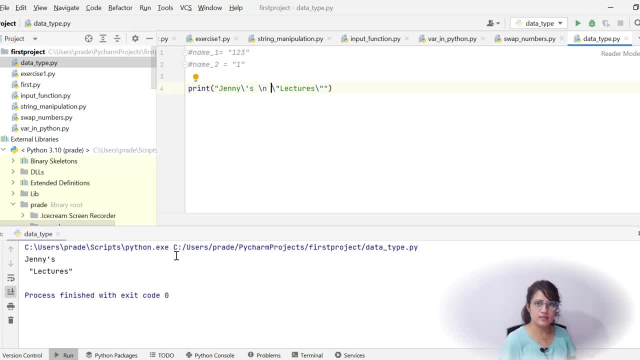 this. so it will show jenny's and lectures in next line. so slash n means new line. it will add new line. yeah, slash n is having a special meaning: escape sequence, escape character is there, but I wanna print, as it is, jenny's slash n lectures. I wanna skip. 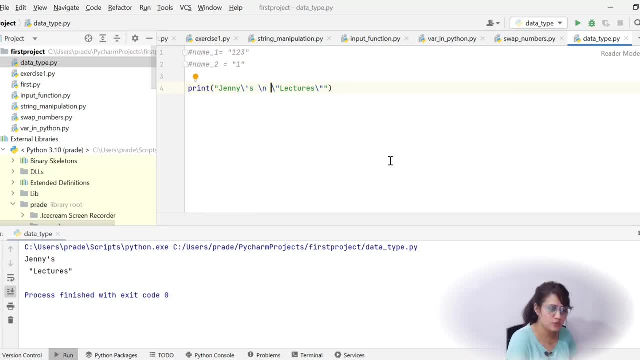 this special meaning of slash n how to skip. just use before this slash n, just use a backslash. so now let's run this and it will print jenny's slash n lectures. ok, I hope you got this way also. ok, skipping of this special meaning of anything and suppose, if you want to print, 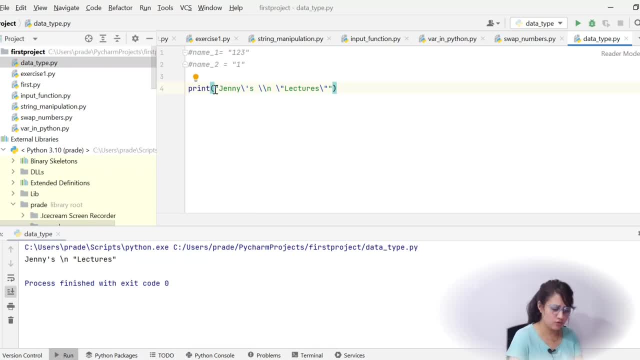 10 times or 5 times. we can do 5 into whatever string you want to print 5 into that and just run this and it will be printed 5 times. that is also possible. I guess you can do these things with strings. so basic is, I guess, clear to you about int float string, how to use. 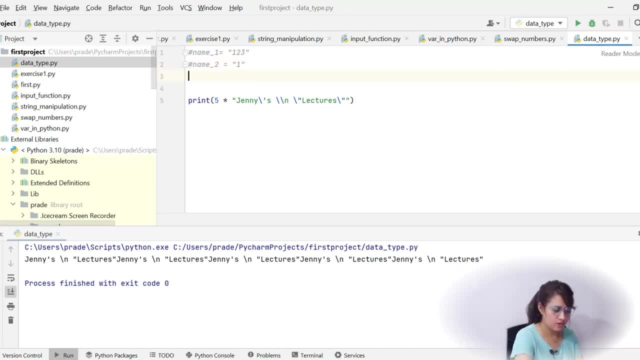 them. and bool is also one more thing. so if I write like variable is equal to if I write c. Take care, this thing, t r u e suppose I am writing. sorry, t r u e true. so rather than this, I wanna print var. so what it will print. let's run this and see what it will print. 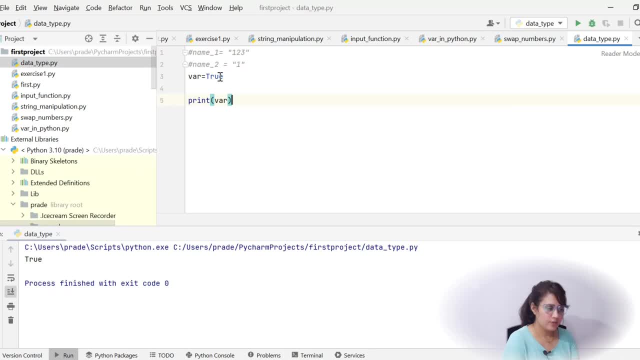 it is printing, true. and if I print this type of this type of this variable var, let's run this. and if the type would be bool, Ok, Ok, Ok, Ok, So see class bool. but if you write t, then it will give error. let's run this and see. 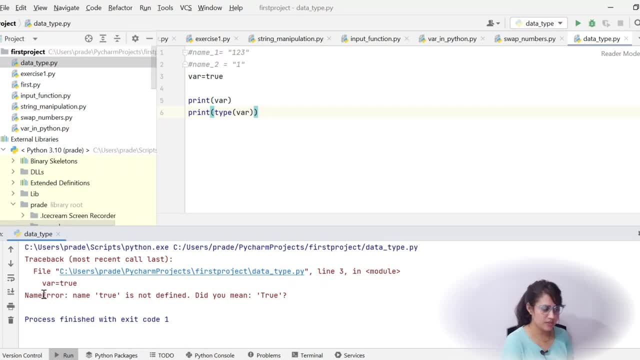 it is a name error. it is a name error, not syntax error, not type error. it is a name error because true and false these are of boolean type, but T F- you have to take care of this thing, but here I am writing t, so it is a name error. name true is not defined. 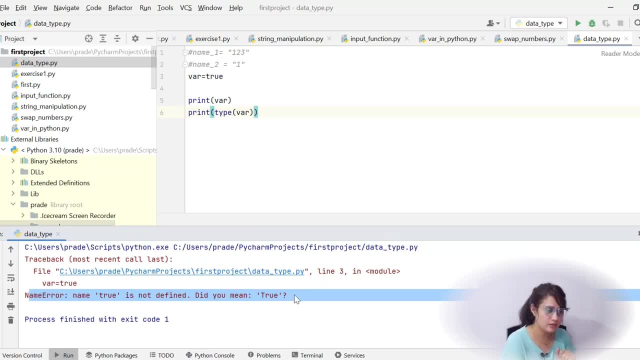 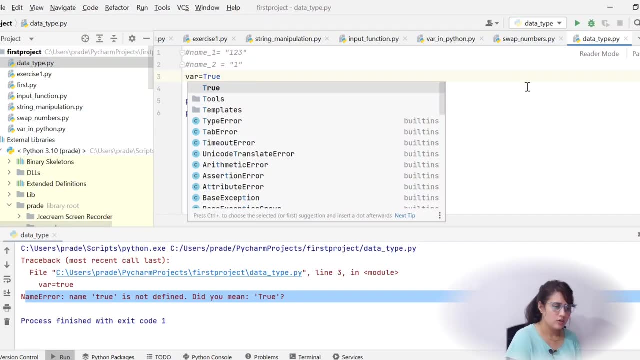 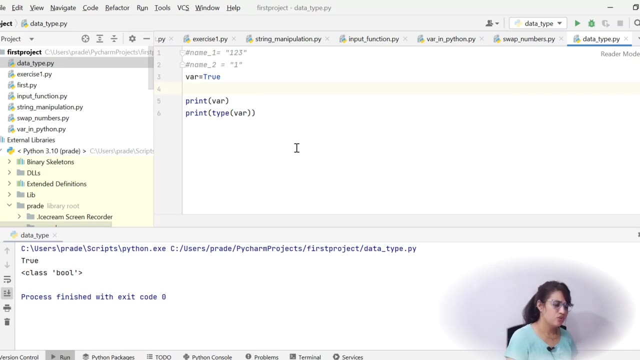 did you mean true, with capital T? yeah, you mean capital T. so here you have to write capital T or you can write false also, and I guess true and false will. you know, will be seeing these thing also in later videos many times we will use when we check any condition.